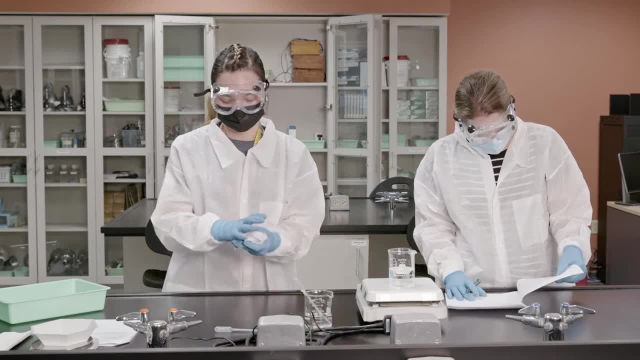 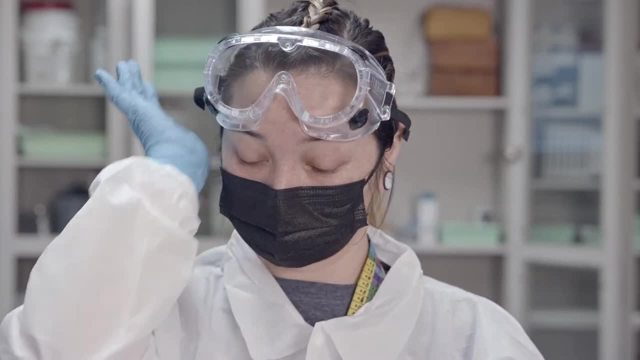 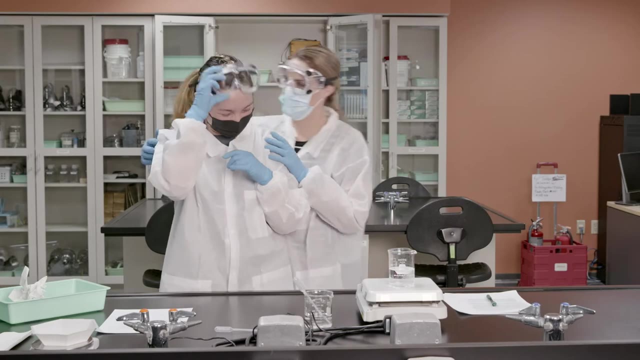 lab. Also, never touch your eyes while in the lab, as your hands may be contaminated with a chemical. In the event that a chemical or hazardous liquid does get into your eyes, proceed immediately to the nearest eyewash station. It may be difficult to see, so ask someone for help. Most eyewash stations have a lever or 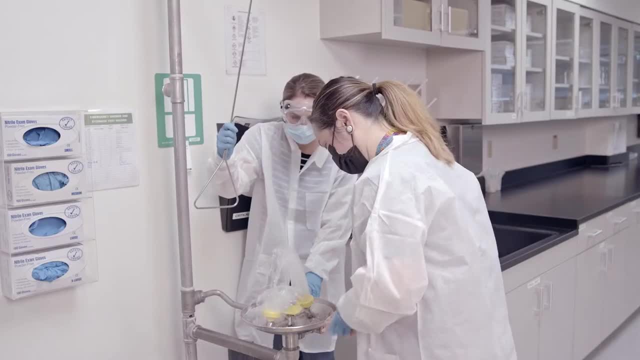 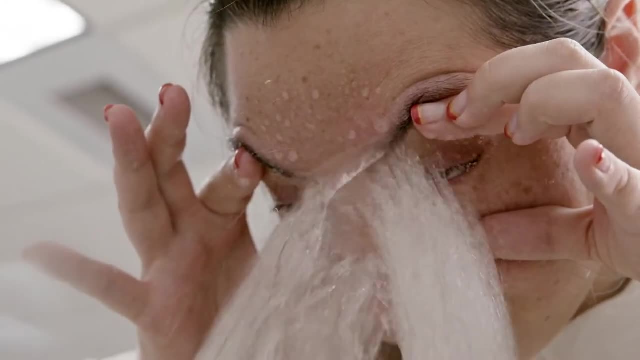 handle to activate the water flow. Activate the water flow and place your eyes directly in the water. You will need to hold your eyelids open and let the water wash your eyes for 15 minutes. It will not be comfortable to hold your eyes open in the water for that long, but it is necessary to flush out the 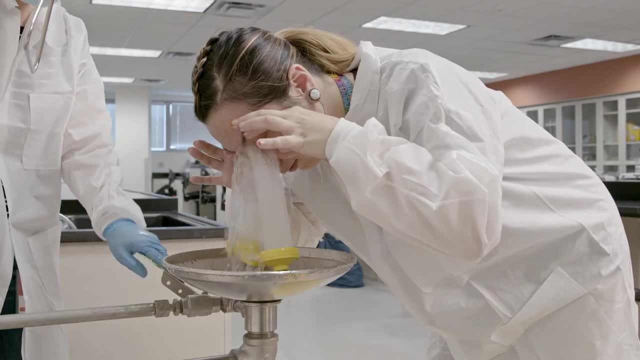 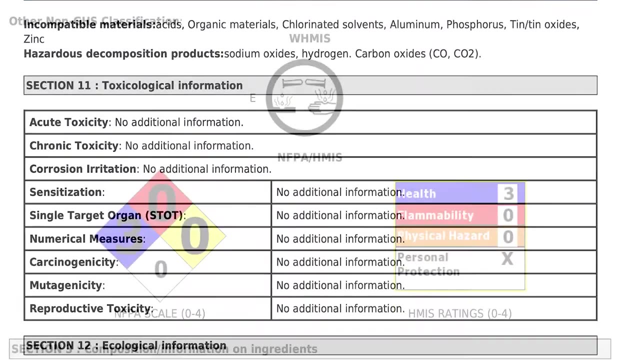 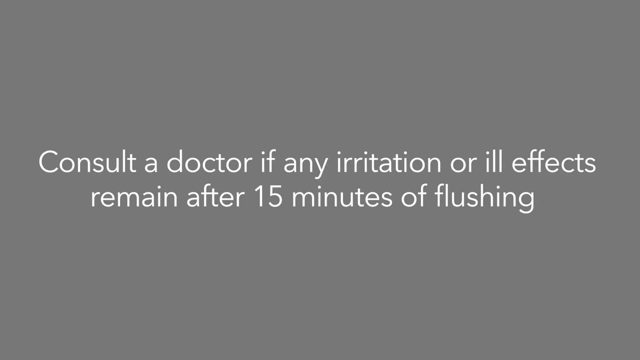 hazardous material and it is well worth it to save your eyes. Have someone call security and check the SDS for the material that was splashed in your eyes. Ensure that security documents the incident with an incident report. afterward Consult a doctor if any irritation or ill effects remain after. 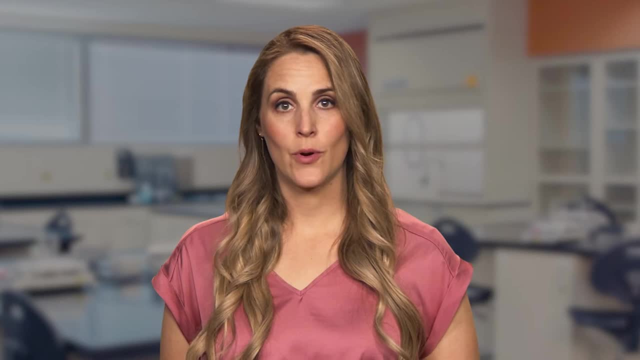 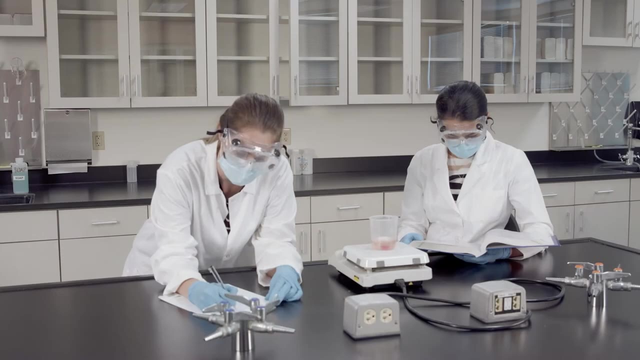 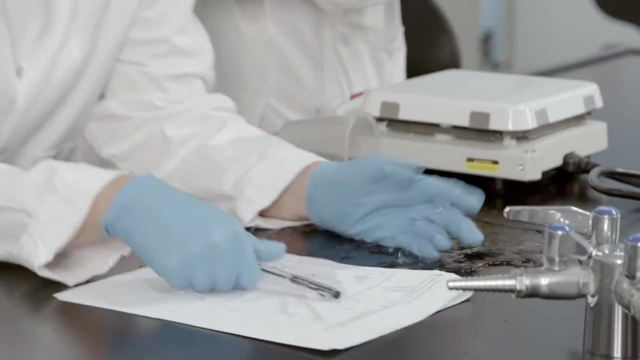 15 minutes of flushing. It is possible that you will spill a chemical or hazardous material on your skin in the lab, especially if you're not wearing protective sleeves or a lab coat. Depending on your campus or your course, lab coats may or may not be required In the event of a small splash to your arms. 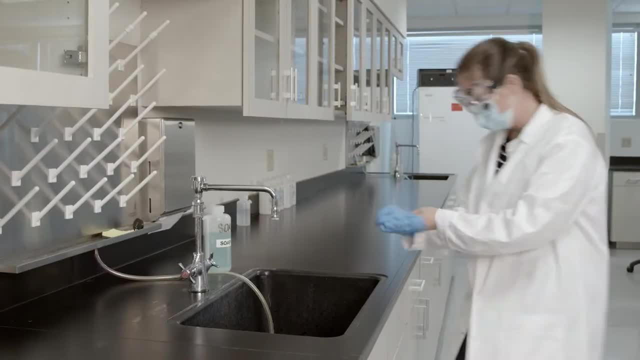 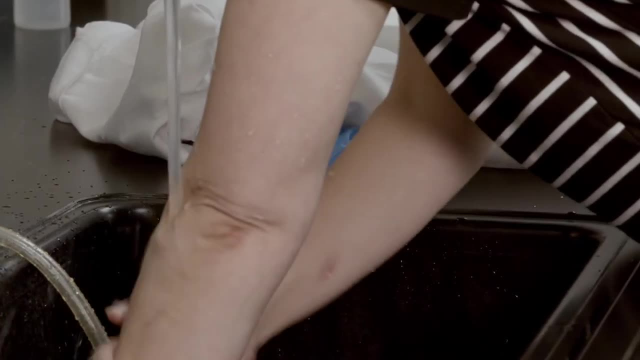 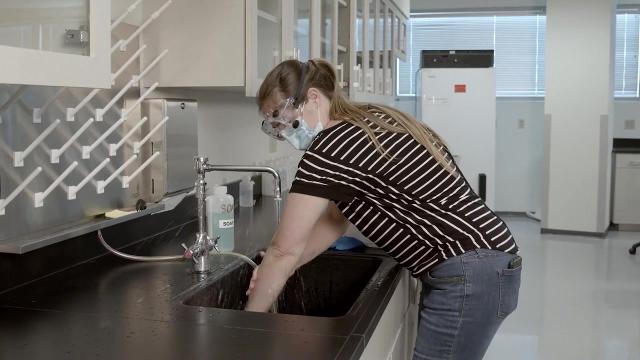 or hands. you should remove your lab coat and go to the nearest sink to flush your skin with water for 15 minutes. Have someone check the SDS to determine if any further action is required based on the chemical or hazardous material, and have someone call security to any exposure of a chemical or hazardous 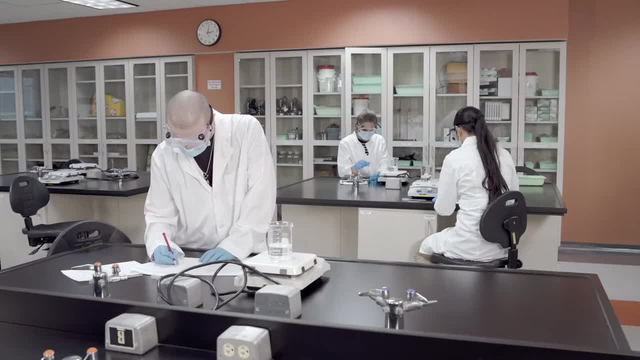 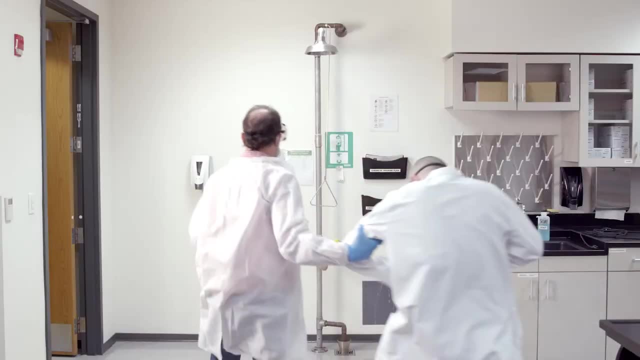 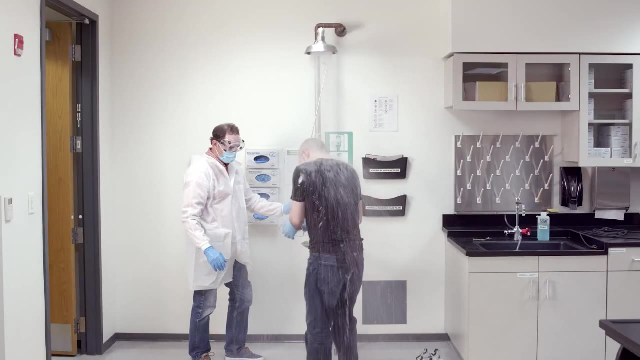 material to document the incident with an incident report. If a chemical spill occurs over a large portion of the body, it will be necessary to use the safety shower. Move immediately to the shower and begin removing contaminated clothing. If you are in the lab with someone who needs to use the shower, assist them Let. 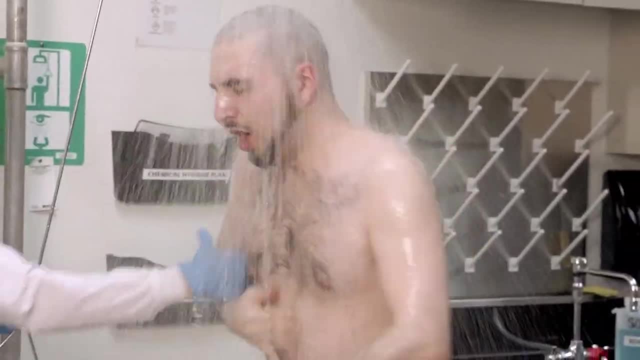 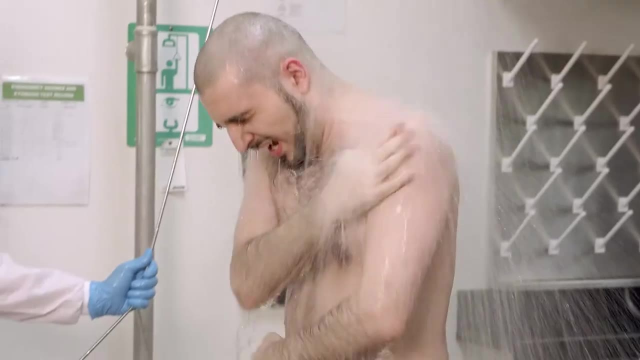 the water flow for 15 minutes to fully rinse your skin to remove the hazardous material. Now is not the time for modesty. You will want to remove all the hazardous material from your body. Have someone check the SDS to determine if any further action is required, based on.